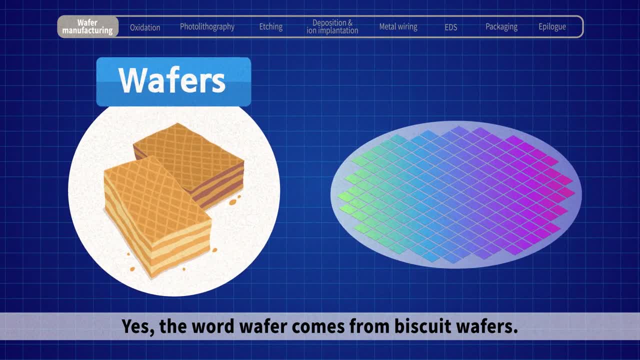 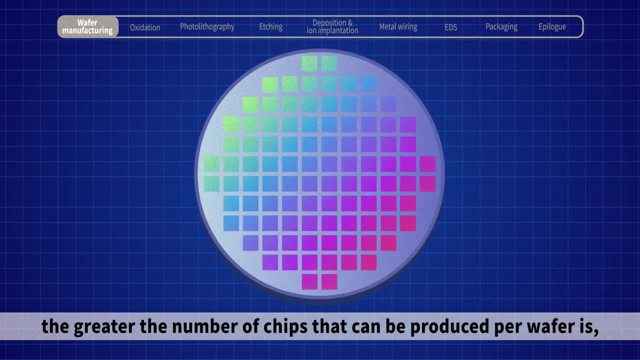 Yes, the word wafer comes from biscuit wafers. A wafer made this way is the main material for semiconductors, Because the larger the diameter is, the greater the number of chips that can be produced per wafer is. 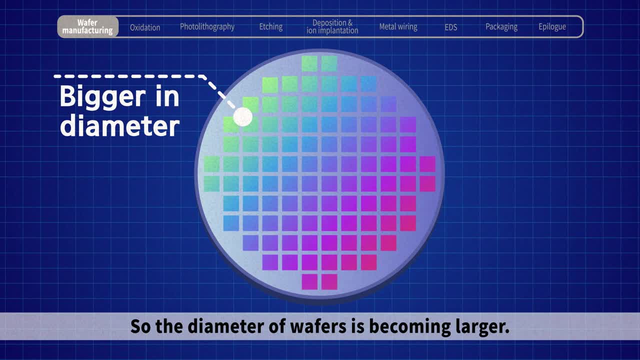 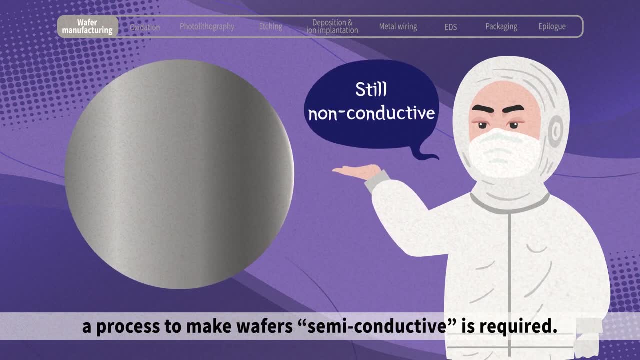 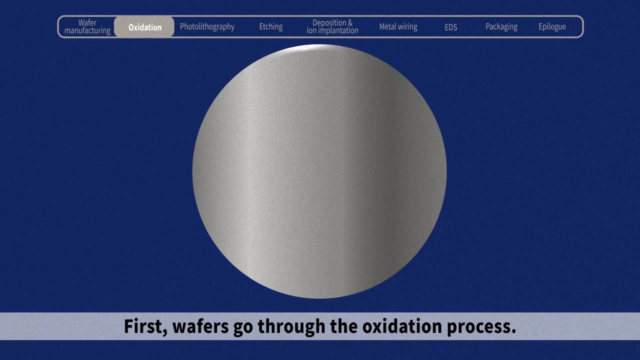 So the diameter of wafers is becoming larger, Because the resultant thin, disc-shaped wafer is not conductive. yet a process to make wafers semi-conductive is required. First wafers go through the oxidation process. 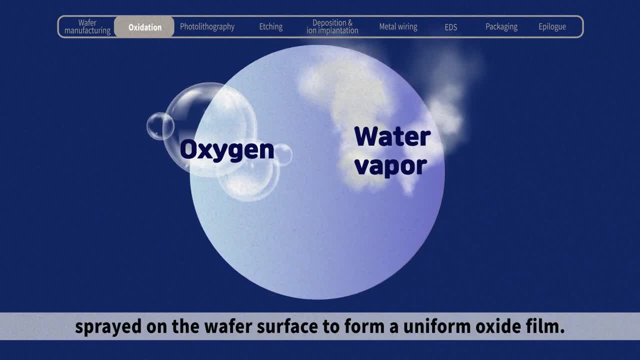 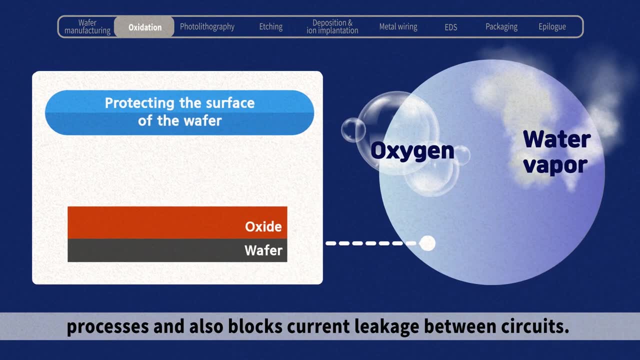 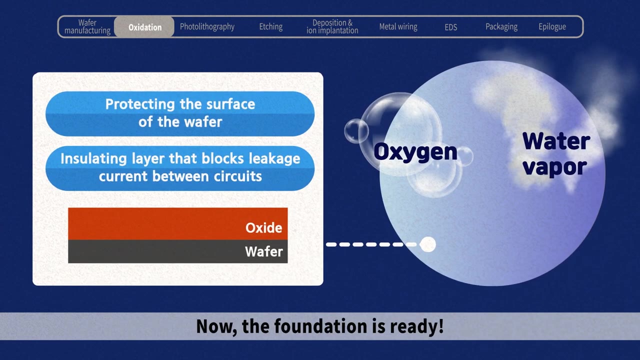 Oxygen or water vapor is sprayed on the wafer surface to form a uniform oxide film. This oxide film protects the wafer surface during the following processes and also blocks current leakage between circuits. The film acts as a strong protective shield. Now the foundation of the wafer is the silicon rod. 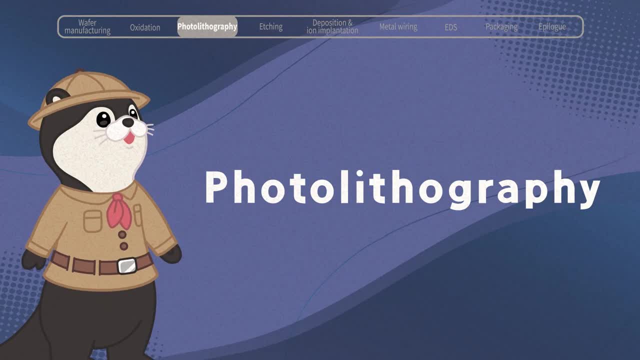 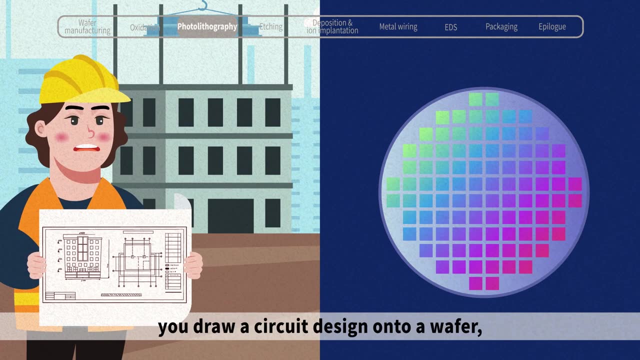 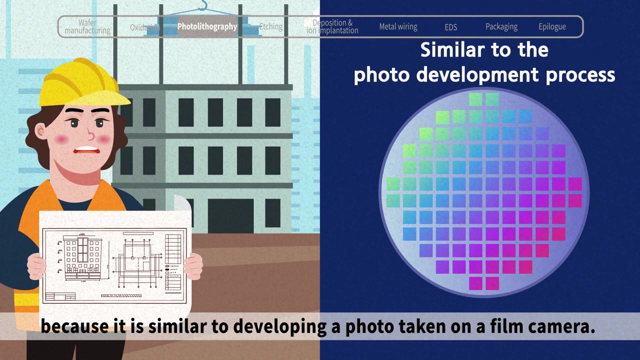 The foundation is ready, The building up process begins. Just as you draw blueprints to build a building, you draw a circuit design onto a wafer, which is called the photolithography process. It is called photo for short because it is similar to developing a photo taken on a film camera. 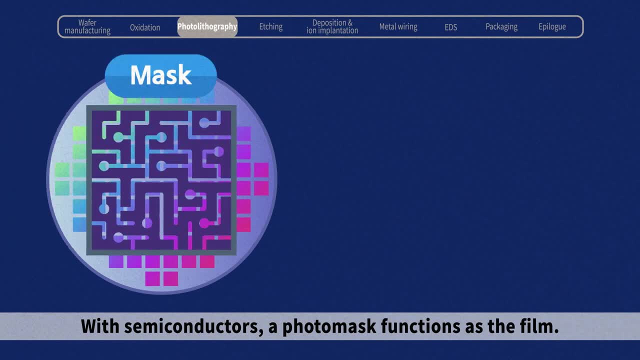 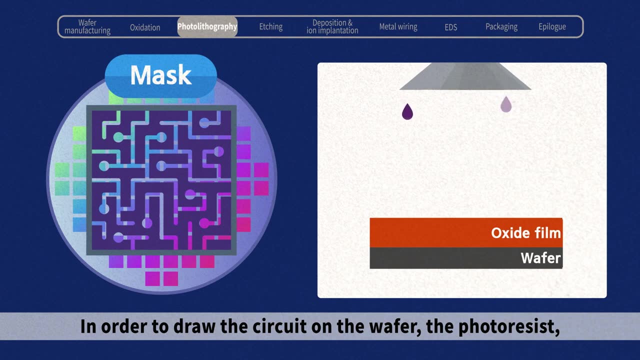 With semiconductors. a photo mask functions as the film. A photo mask is a glass substrate with a computer-designed circuit pattern. In order to draw the circuit on the wafer, the photo resist, a material that responds to light, is applied thinly and evenly on the oxide film previously placed on the wafer. 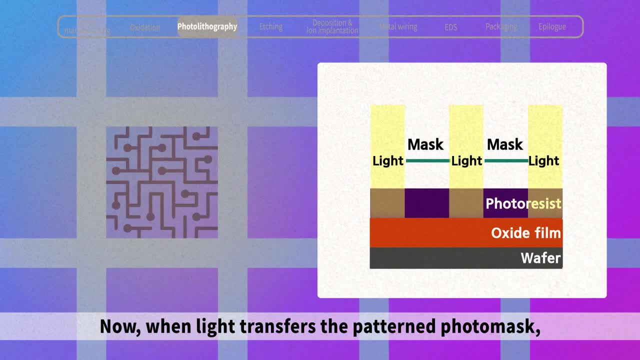 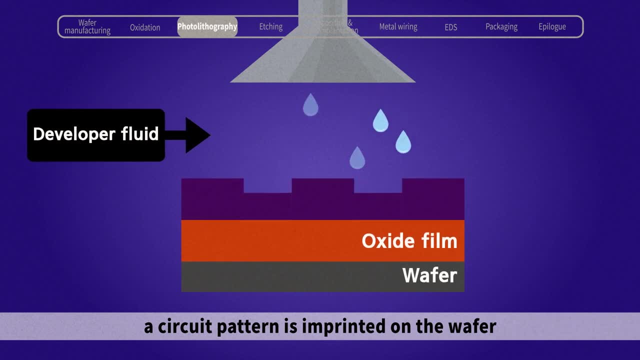 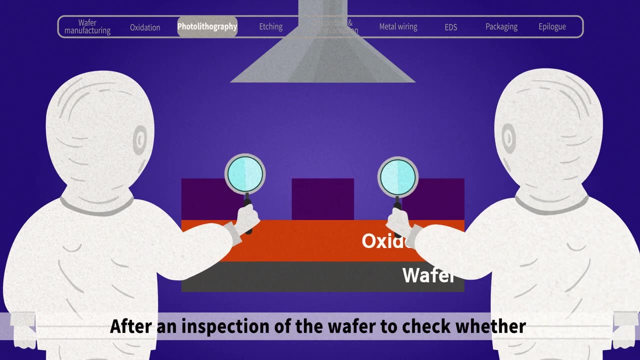 Now, when light transfers the patterned photo mask, the circuit is drawn on the wafer surface. Just like developing a photo, a circuit pattern is imprinted on the wafer by spraying, developer and removing unlit areas from the areas that are exposed to light. After an inspection of the wafer, 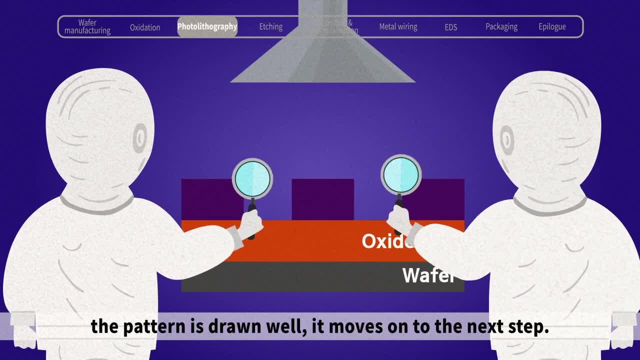 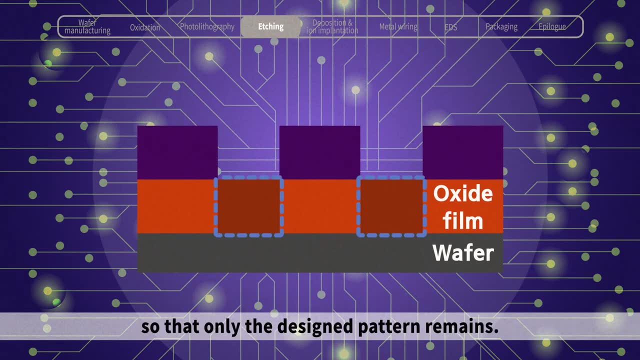 to check whether the pattern is drawn well, it moves on to the next step. Now unnecessary materials are carved out so that only the design pattern remains. Using a liquid or gas etching, unnecessary materials are selectively removed to draw the desired design. 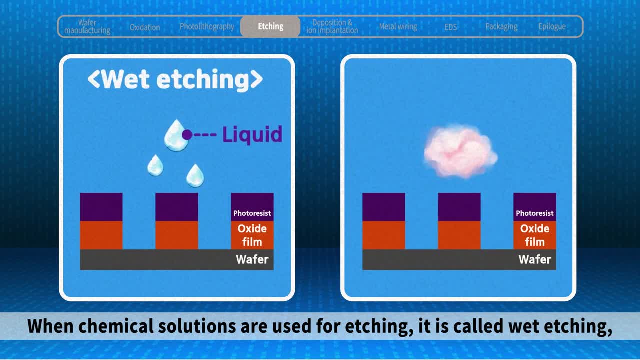 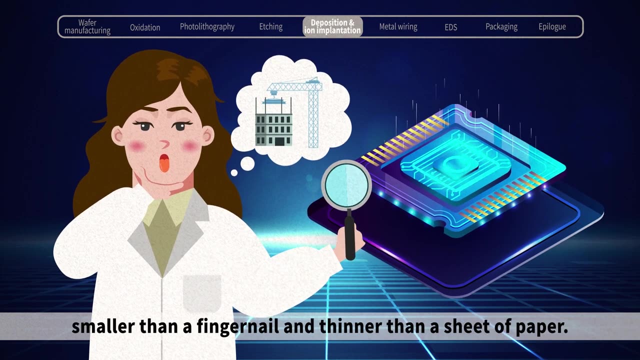 When chemical solutions are used for etching, it is called wet etching, And when gas or plasma is used, it is called dry etching. We will talk about these details in the future. Let's imagine constructing a building on a semiconductor chip smaller than a fingernail. 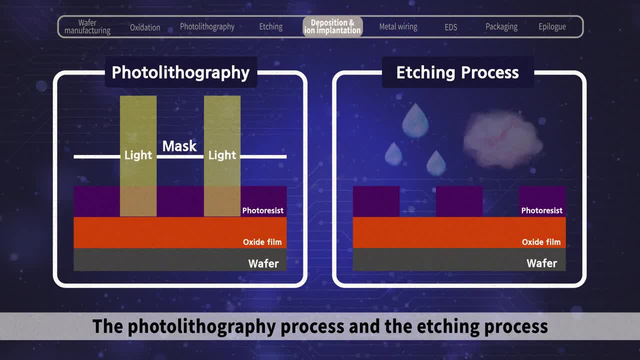 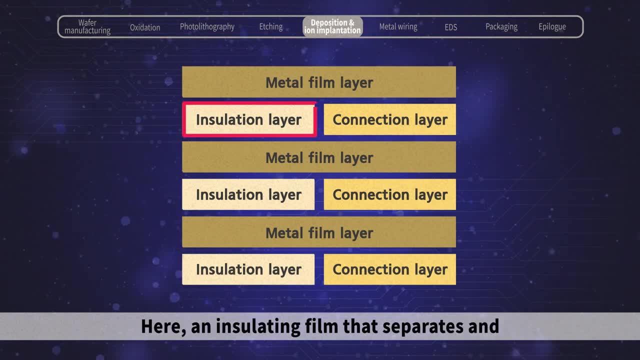 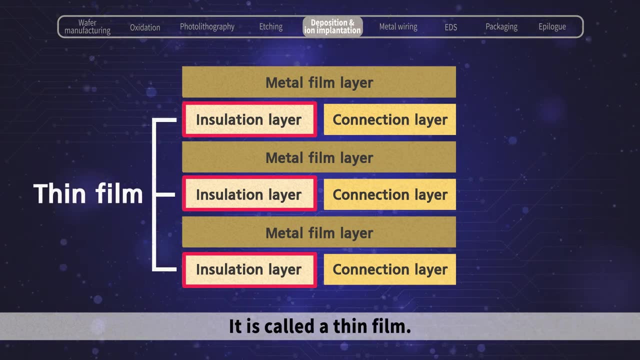 and thinner than a sheet of paper. The photolithography process and the etching process are repeated several times on the wafer, layer by layer. Here, an insulating film that separates and protects the stacked circuits is required. It is called a thin film. 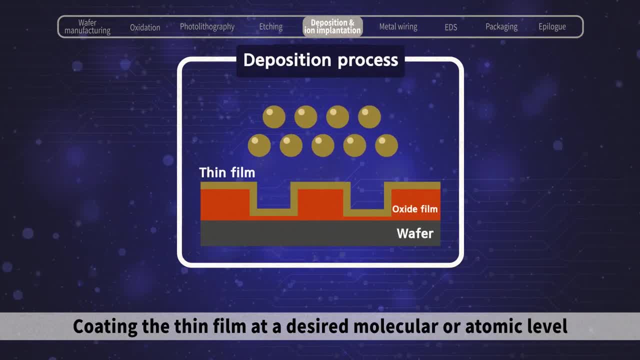 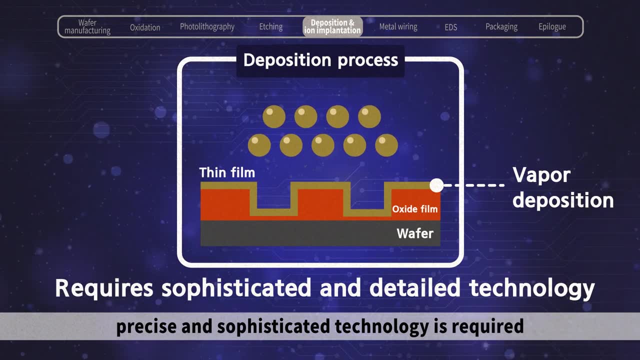 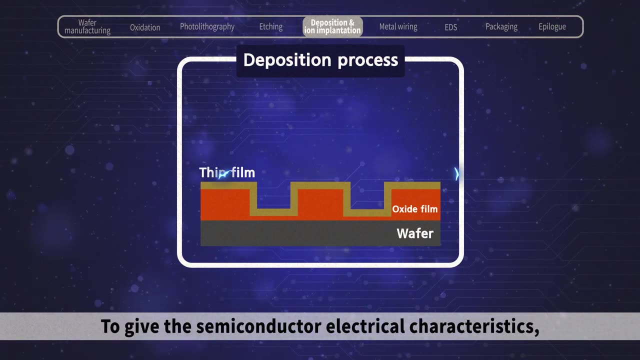 Coating the thin film at a desired molecular level or atomic level onto a wafer is called deposition. Since the coating is so thin, precise and sophisticated technology is required to uniformly apply the thin film on a wafer To give the semiconductor electrical characteristics. 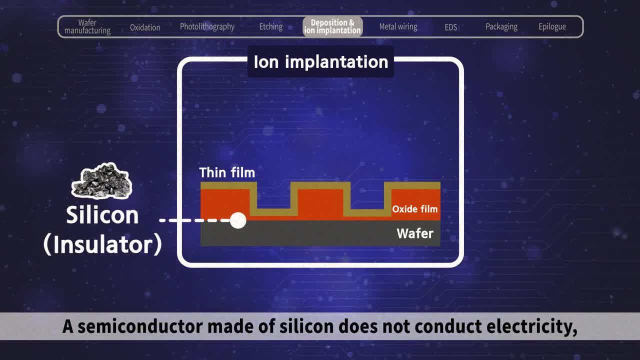 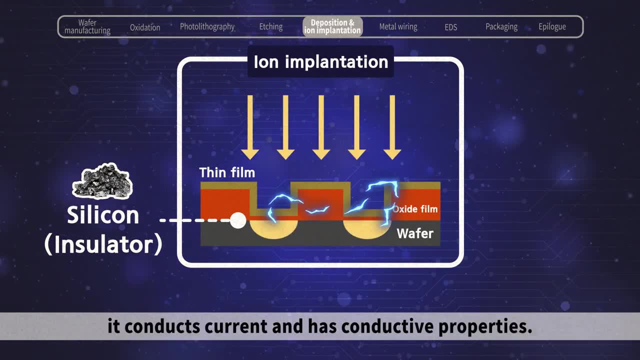 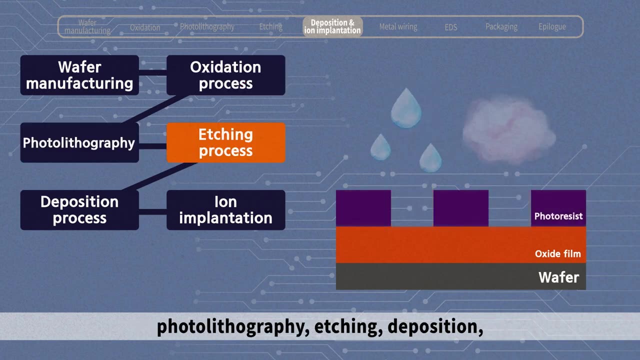 ion implementation is also required. A semiconductor made of silicon does not conduct electricity but adding impurities, it conducts current and has conductive properties. In summary, through the wafer manufacturing, oxidation, photolithography, etching, deposition and ion implementation processes. 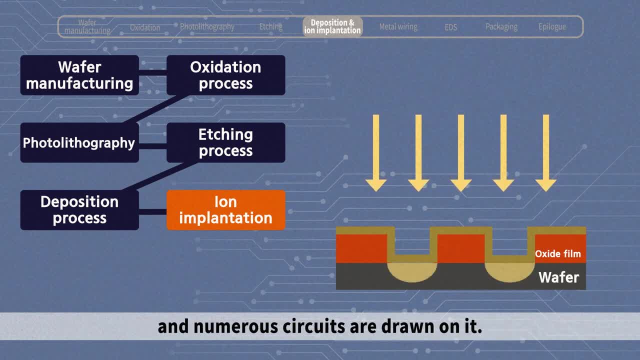 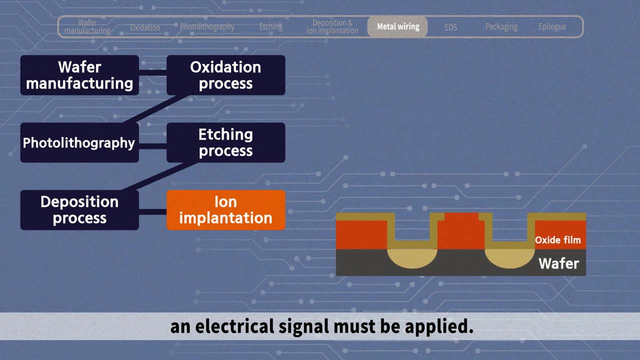 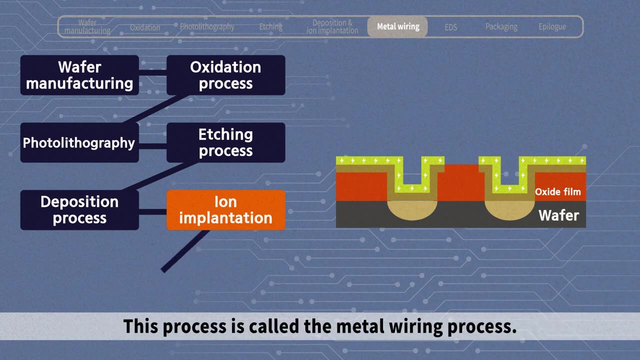 the wafer becomes conductive and numerous circuits are drawn on it. Now, in order for this circuit to work, an electrical signal must be applied. It is necessary to create a path for electricity to pass through according to the circuit pattern. This process is called the metal wiring process. 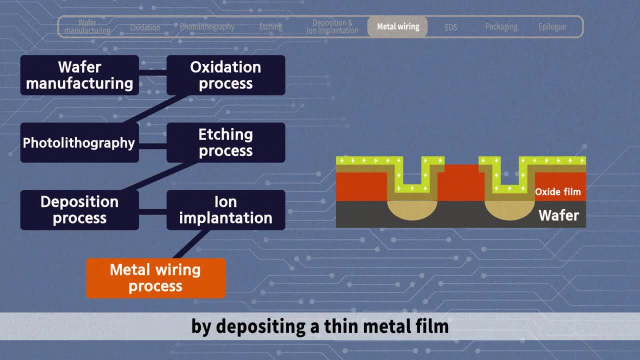 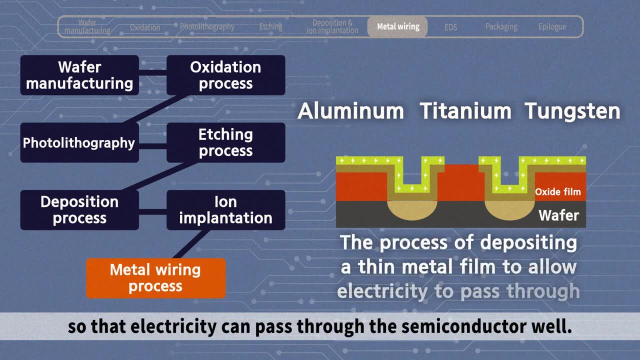 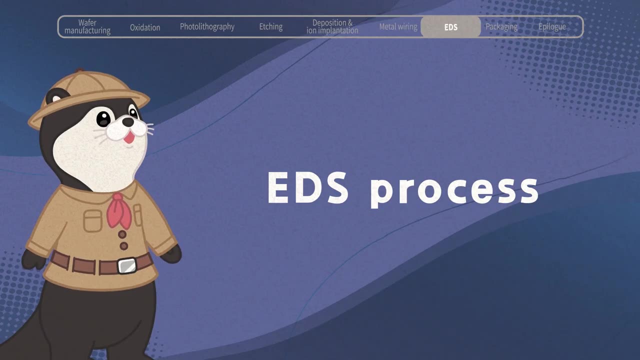 It is a process that allows electricity to flow by depositing a thin metal film, using materials such as aluminum, titanium or tungsten, so that electricity can pass through the semiconductor. well, The chip manufacturing processes are now coming toward completion. The next step is EDS. 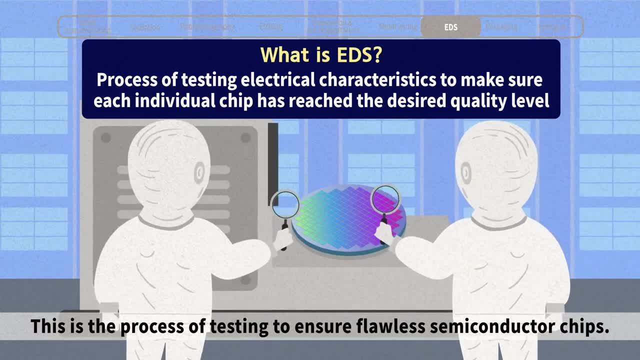 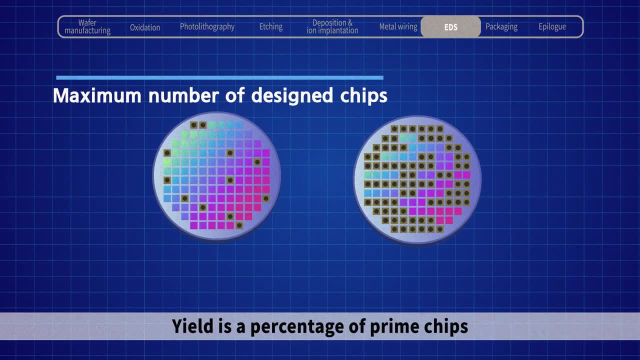 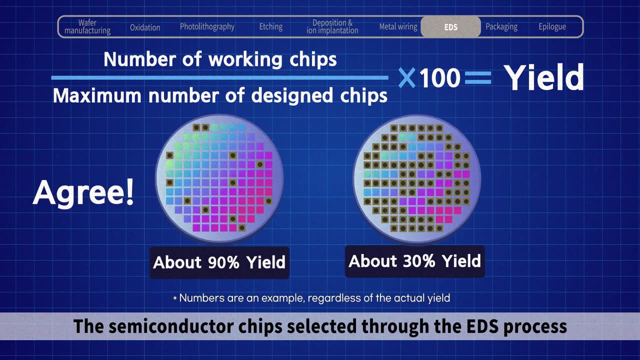 This is the process of testing to ensure flawless semiconductor chips. In other words, it is a testing step to sort out defective chips. Yield is a percentage of prime chips relative to the maximum chip count on a single wafer. The semiconductor chips selected through the EDS process. 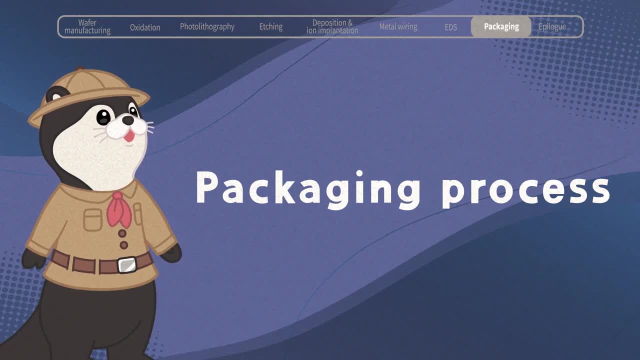 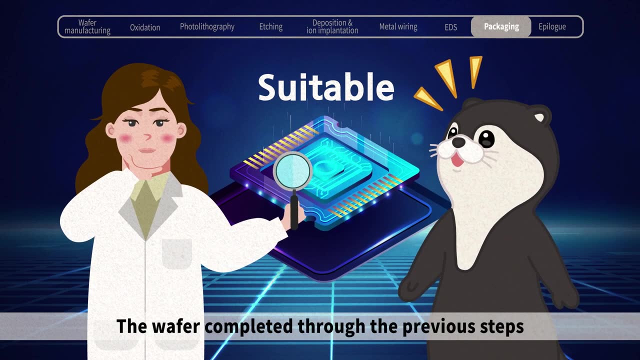 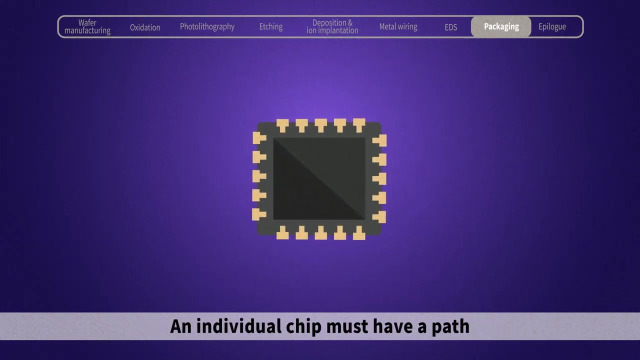 are made in a form suitable for devices. This is the last process, the packaging process. The wafer completed through the previous steps are cut into individual semiconductor chips that can be loaded on an electronic device. An individual chip must have a path to exchange electrical signals with the outside.